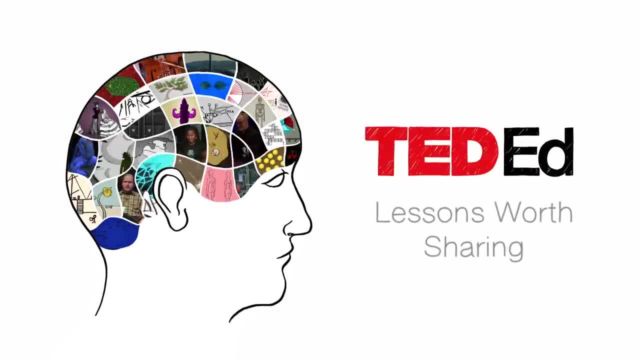 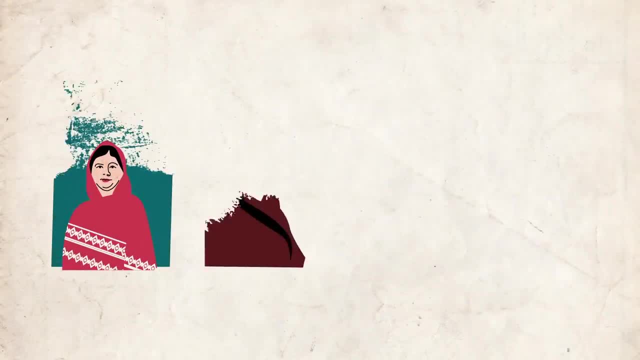 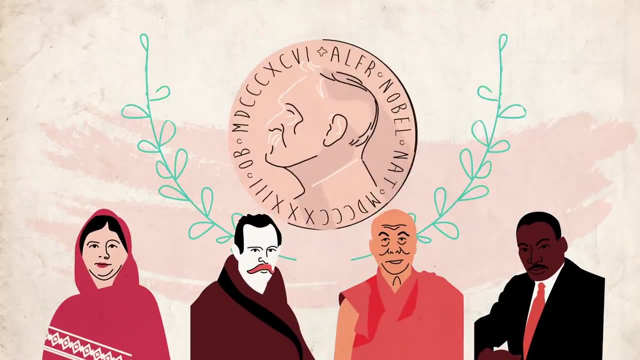 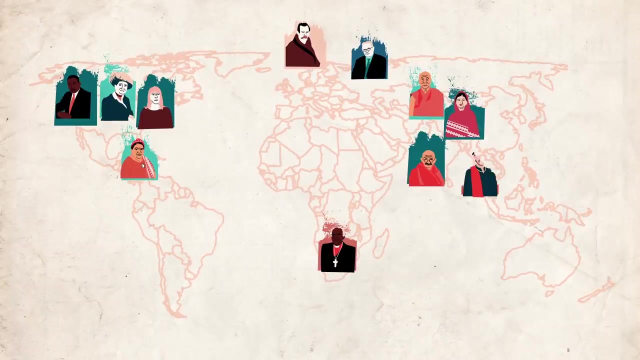 What do a 17-year-old Pakistani, a Norwegian explorer, a Tibetan monk and an American pastor have in common? They were all awarded the Nobel Peace Prize. Among the top, prestigious awards in the world, this prize has honored some of the most celebrated and revered. 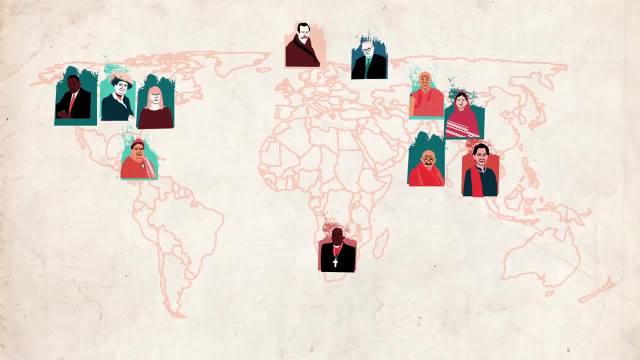 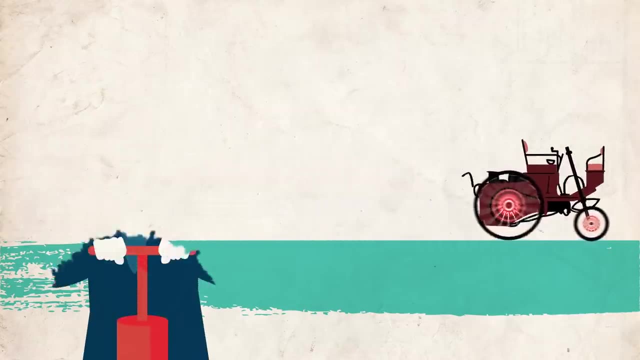 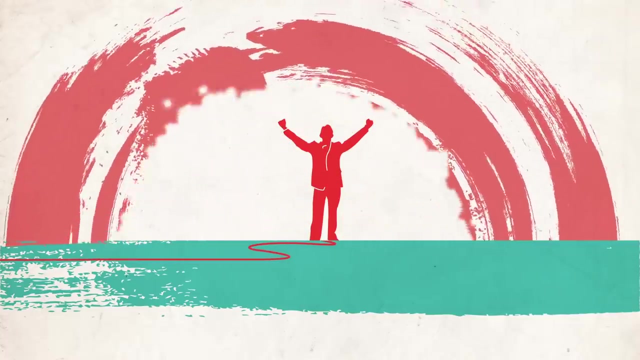 international figures and organizations in history. To understand how it all got started, we have to go back to the 1800s. Swedish chemist Alfred Nobel was then mostly known for the invention of dynamite, a breakthrough which launched his career as a successful inventor and businessman. 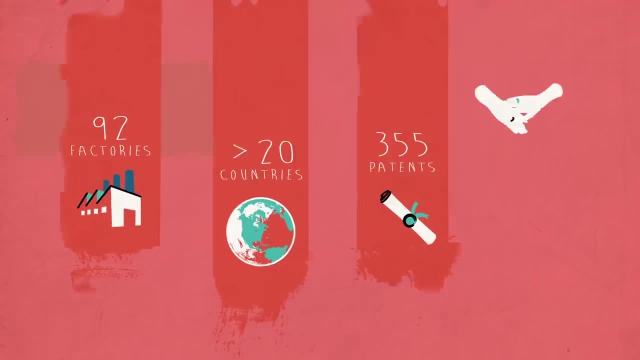 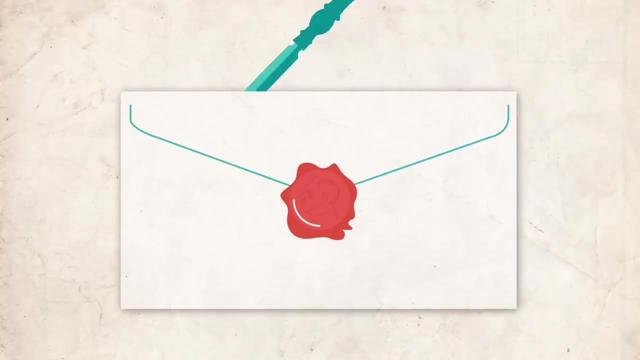 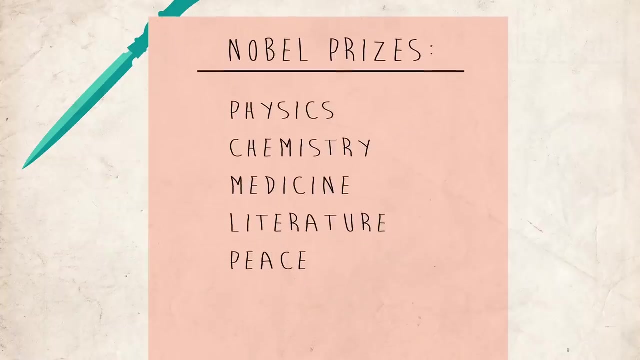 Thirty years later, he had become extremely wealthy but never married and had no children. When his will was opened after his death, it came as a surprise that his fortune was to be used for five prizes in physics, chemistry, medicine, literature and peace. 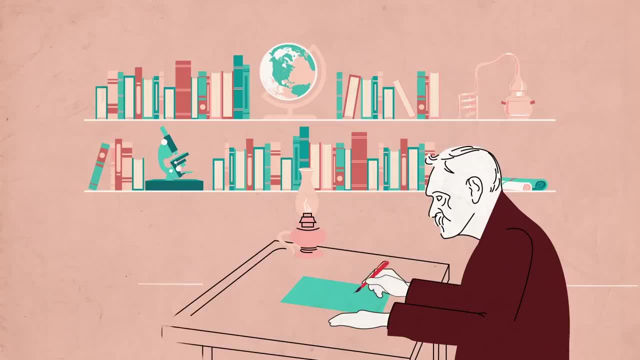 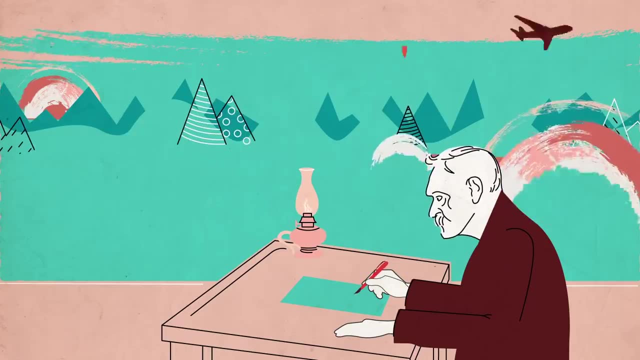 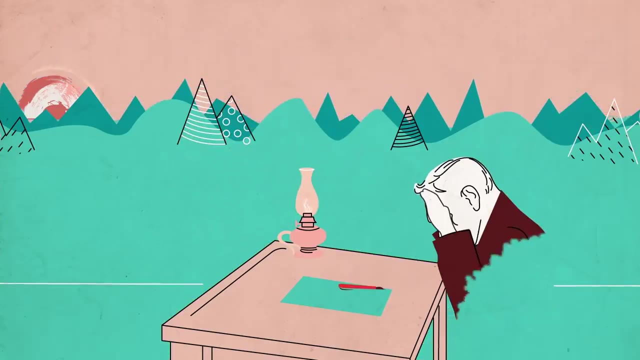 These prizes illustrated his lifelong commitment to sciences and his passion for literature. But what about peace? Because Nobel's name was tied to inventions used in the war industry, many have assumed that he created the Peace Prize out of regret. However, this is all speculation. 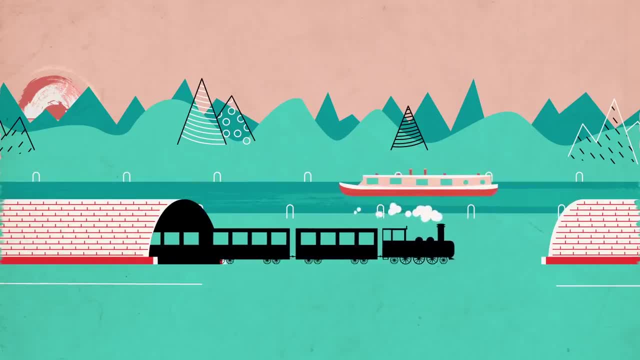 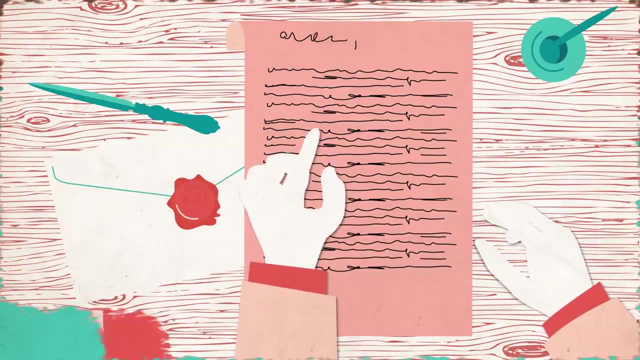 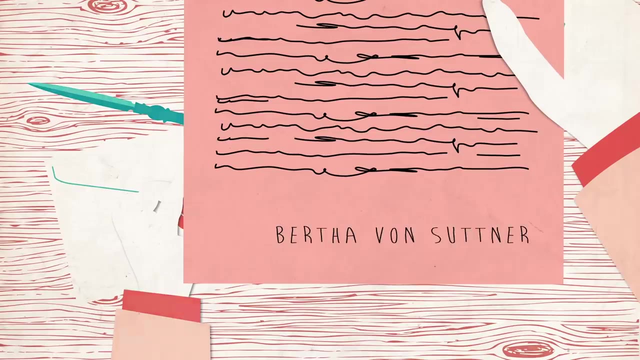 as he never expressed any such sentiments, and his inventions were also used for constructive purposes. Instead, many historians connect Alfred Nobel's interest for the peace cause to his decade-long friendship and correspondence with an Austrian pacifist named Bertha von Züttner. 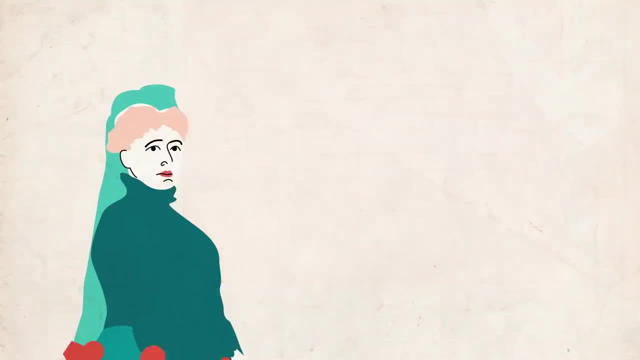 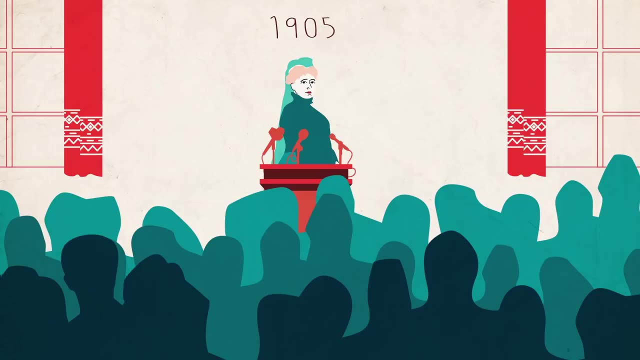 Von Züttner was one of the leaders of the international peace movement and in 1905, after Nobel's death, she became the first woman to be awarded the Nobel Peace Prize. Nobel's will outlined three criteria for the Peace Prize. 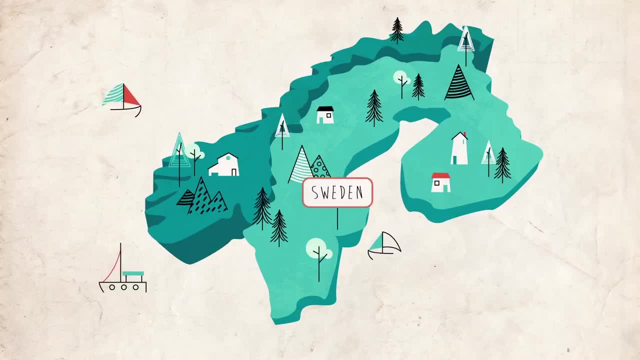 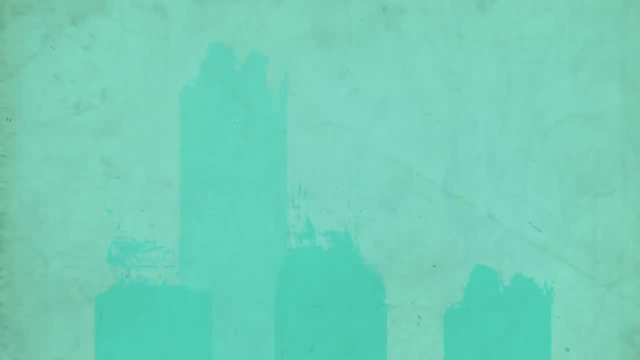 which, unlike the other Sweden-based prizes, would be different. The first criteria would be administered in Norway: disarmament, peace congresses and brotherhood between nations. These standards have since been expanded to include other ways of promoting peace, such as human rights and negotiations. 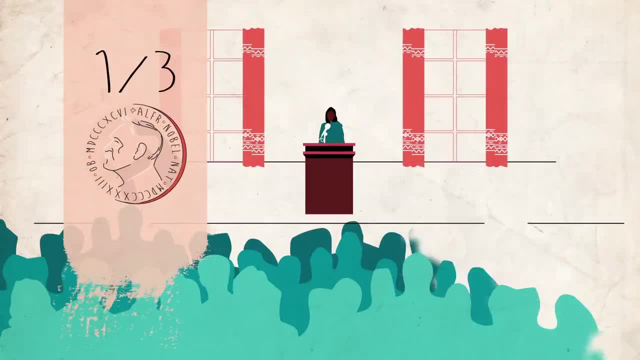 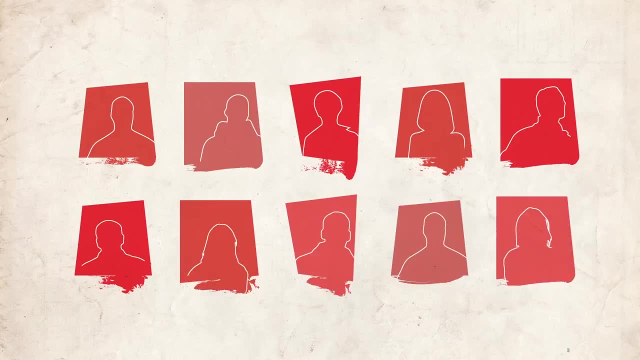 And the prize doesn't just have to go to one person. About a third of Nobel Peace Prizes have been shared by two or three laureates, So how do nominations for the prize work? According to the Nobel Foundation, a valid nomination can come from a member. 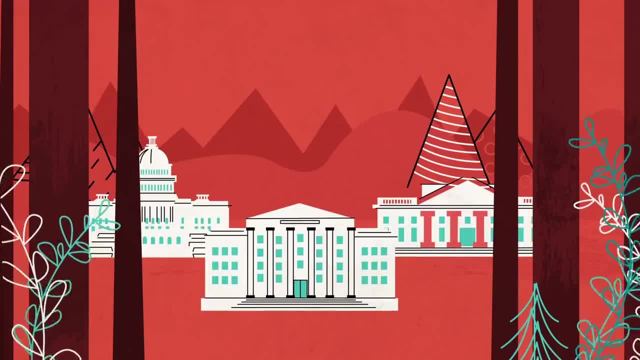 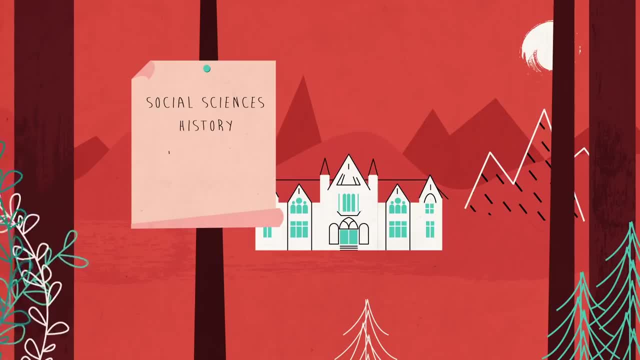 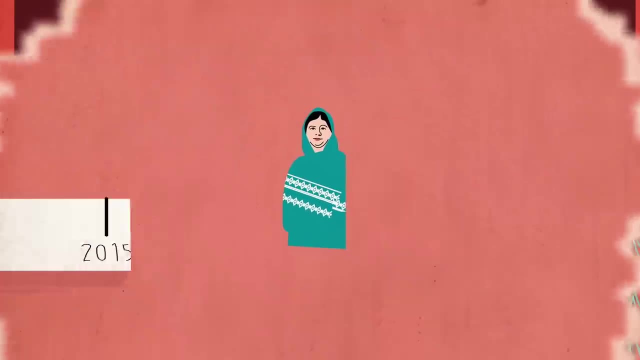 of a national assembly, state government or an international court. Eligible nominators also include university rectors, professors of the social sciences, history, philosophy, law and theology, and previous recipients of the Peace Prize. But if you want to know more about who was recently nominated, 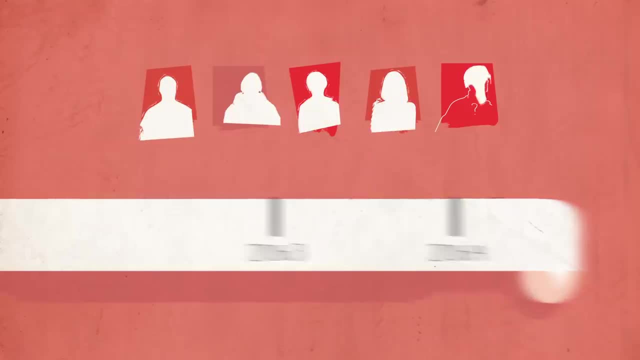 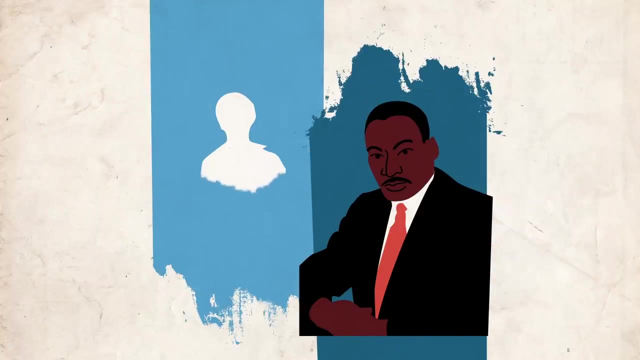 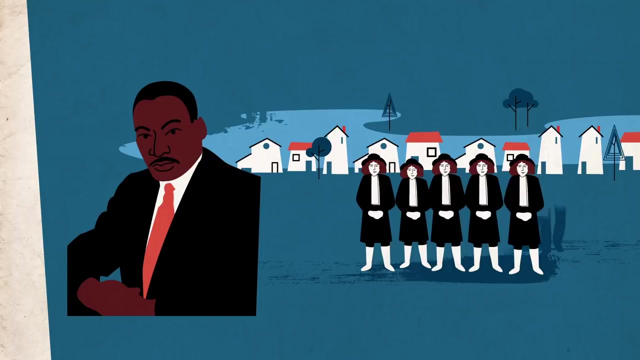 you'll have to be patient. All information about nominations remains secret for 50 years. Take Martin Luther King Jr. We didn't actually know who nominated him until 2014.. His nominators turned out to be the Quakers who had won the prize previously. 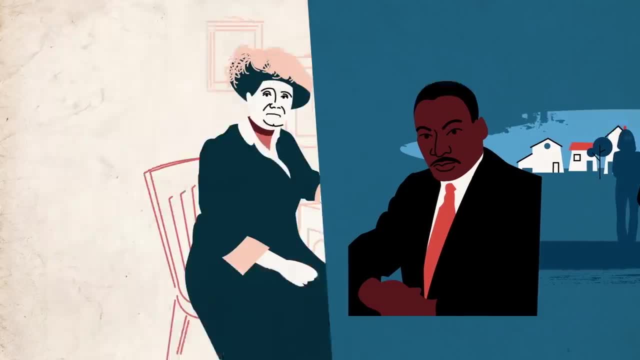 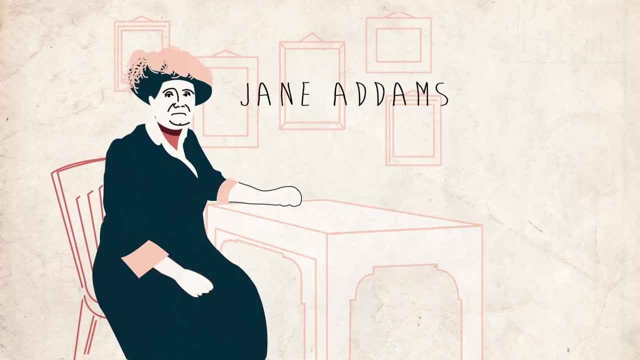 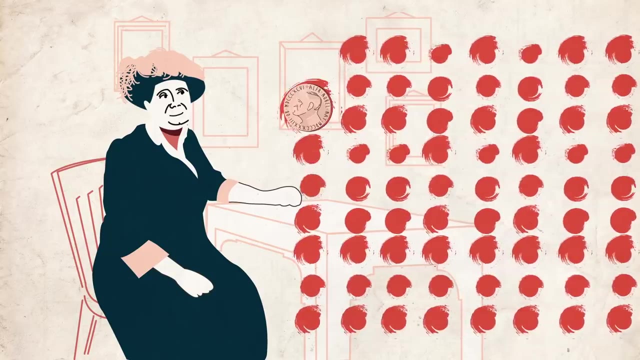 and eight members of the Swedish parliament. There's no limit to the number of times a person or organization can be nominated. In fact, Jane Addams, recognized as the founder of social work in the United States, was nominated 91 times before finally being awarded the prize. 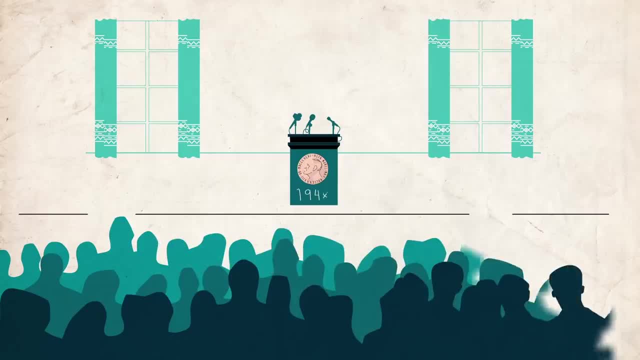 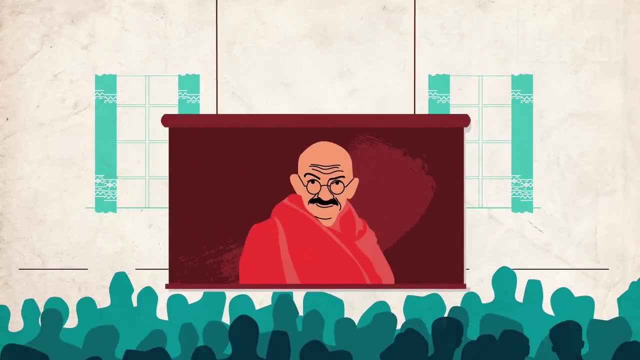 The absence of a laureate can also be symbolic. The 1948 decision not to award the prize following the death of Mahatma Gandhi has been interpreted as an attempt to respectfully honor the so-called missing laureate, As with the other Nobel Prizes. the Peace Prize can't be awarded posthumously. The secret selection process takes almost a year and is carried out by the five appointed members of the Norwegian Nobel Committee, who are forbidden from having any official political function in Norway, Starting with a large pool of nominations. 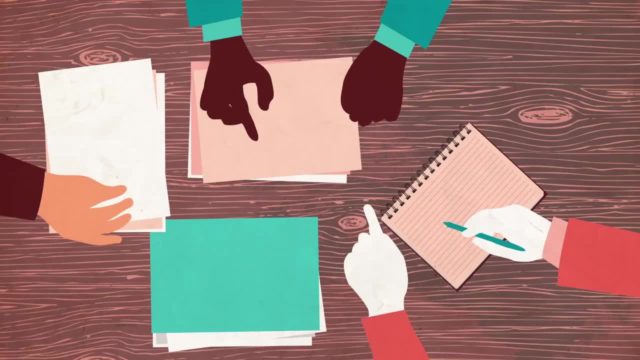 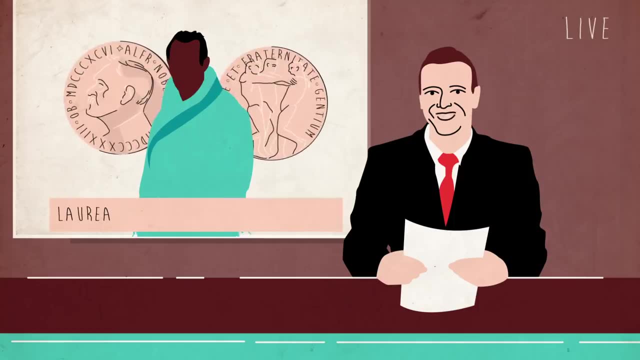 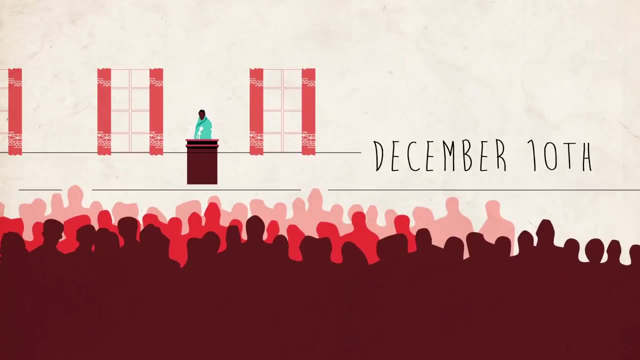 exceeding 300 in recent years. they assess each candidate's work and create a short list. Finally, the chairman of the Nobel Committee publicly announces the laureate in October. The award ceremony takes place on December 10th, the anniversary of Alfred Nobel's death. 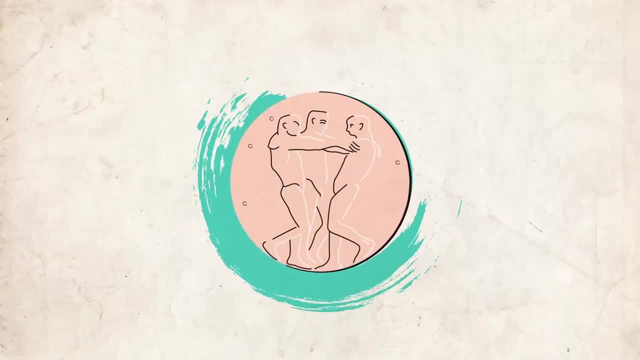 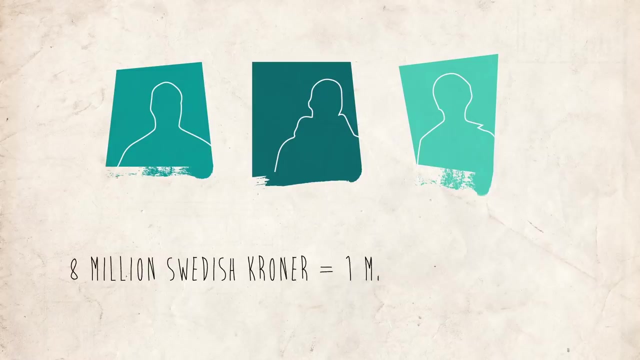 The prize itself includes a gold medal inscribed with the Latin words Propace et Fraternitate Gentium, or For the Peace and Brotherhood of Men, as well as a diploma and a large cash prize. Recently it's been 8 million Swedish kronor. or roughly a million US dollars, which is split in the case of multiple laureates, And while laureates can use the prize money as they choose, in recent years many have donated it to humanitarian or social causes. For many years, the Nobel Peace Prize was predominantly awarded. to European and North American men, But in recent years, significant changes have been taking place, making the prize more global than ever. Twenty-three organizations and 103 individuals, that's 87 men and 16 women, have made up the 126 Nobel Peace Prize laureates in history. 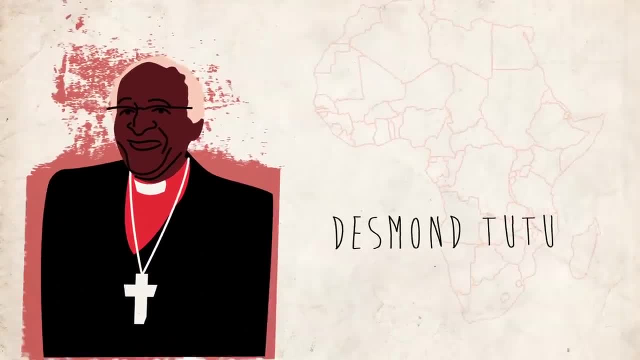 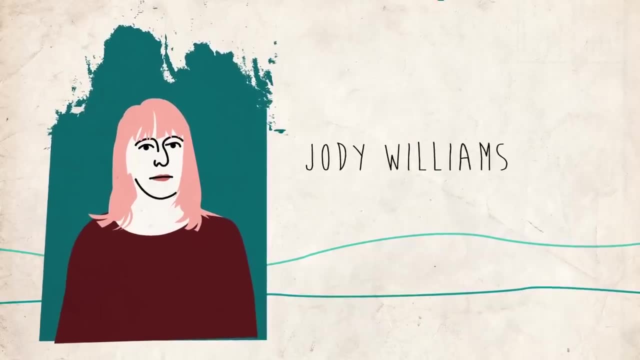 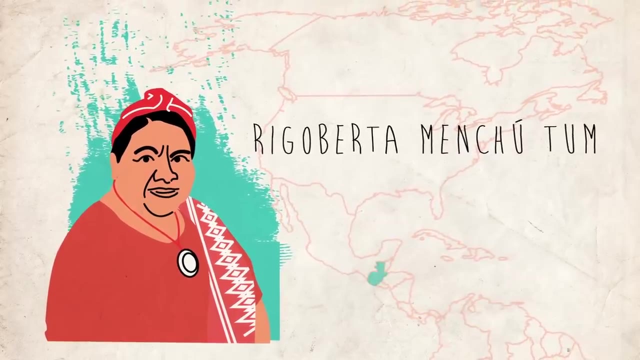 They include Desmond Tutu for his nonviolent campaign against apartheid in South Africa. Jody Williams for her campaign to ban and clear anti-personnel mines. Rigoberta Menchu Tum for her work for social justice and reconciliation based on respect for the rights of indigenous peoples.